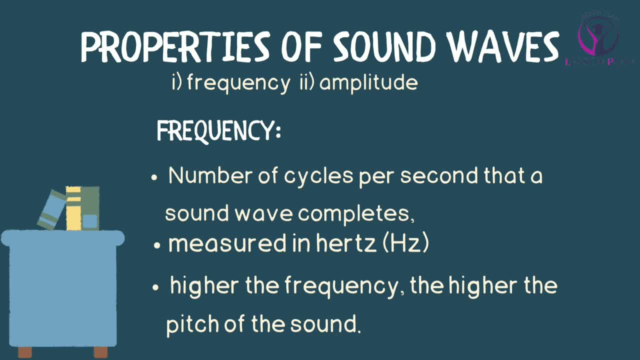 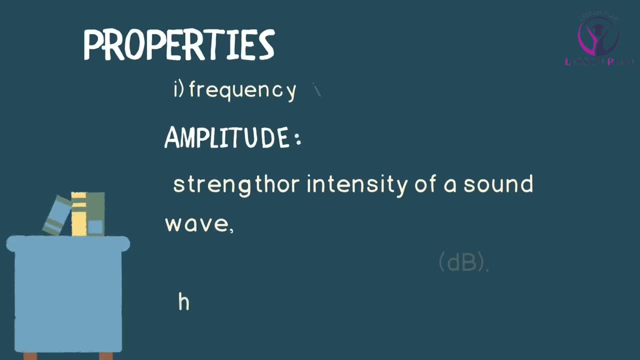 The two main properties we will focus on are frequency and amplitude. Frequency refers to the number of cycles per second that a sound wave completes, and it's measured in Hertz. the higher the frequency, the higher the pitch of the sound. Amplitude refers to the amount of momentum per second that a sound wave completes. Amplitude refers to the value of語, which is equal to the bits on which sound illä in our Choice form and time. Amplitude refer to the number of cycles per second that a sound wave completes, and its measured in Hertz. 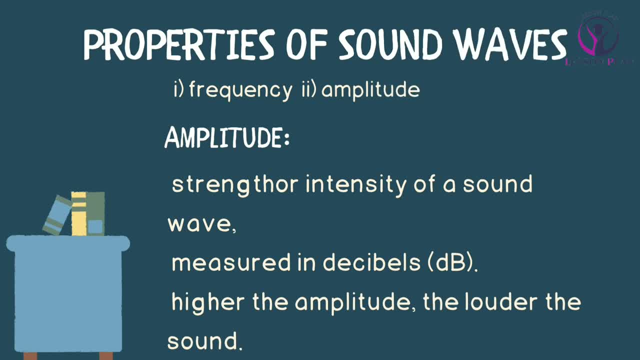 Here the frequency refers to the number of w accepting music or any material. Amplitude refers to the number of Brazil uważataríc. natural Sound waves: the higher the frequent sound. and white Amplitude refers to the strength or intensity of a sound wave, and it's measured in decibels. 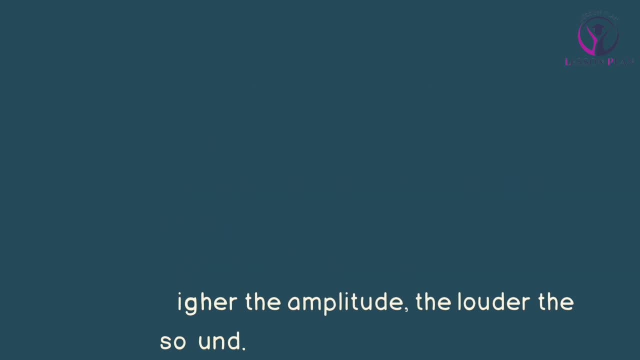 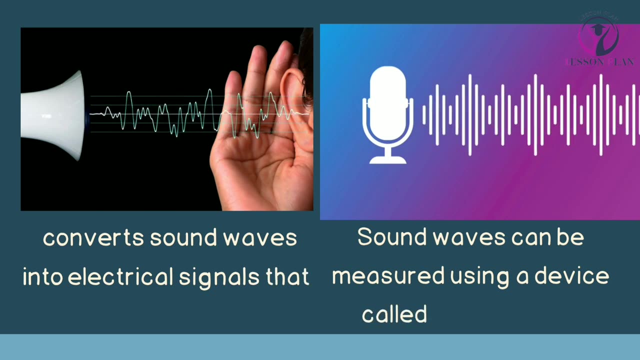 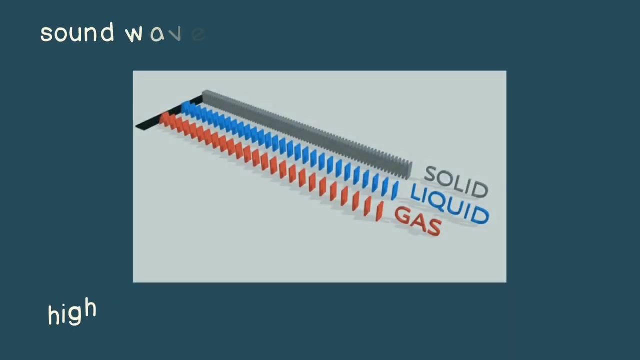 Sound waves can be measured using a device called a microphone, which converts sound waves into electrical signals that can be analyzed. Sound waves can also be created by a variety of sources, such as musical instruments, human voices and even natural phenomena like thunder. 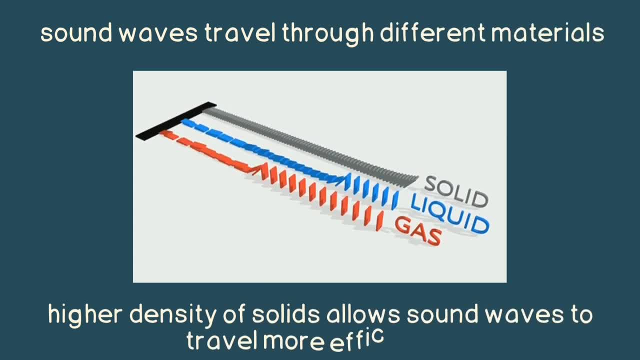 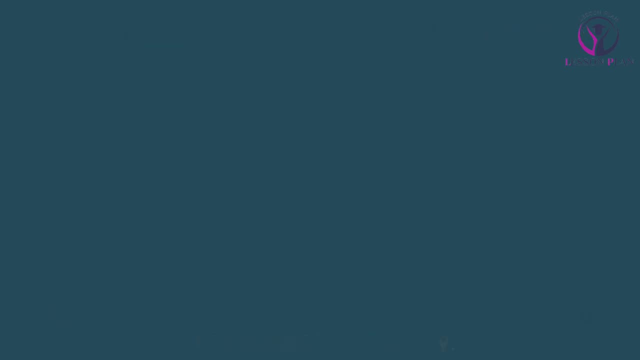 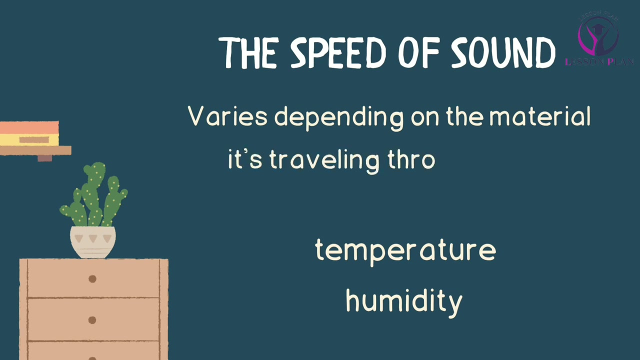 Finally, let's talk about how sound waves travel through different materials. Sound waves travel fastest through solids, followed by liquids and then gases. This is because solids have a higher density, which allows sound waves to travel more efficiently. The speed of sound also varies depending on the material it's traveling through as well. 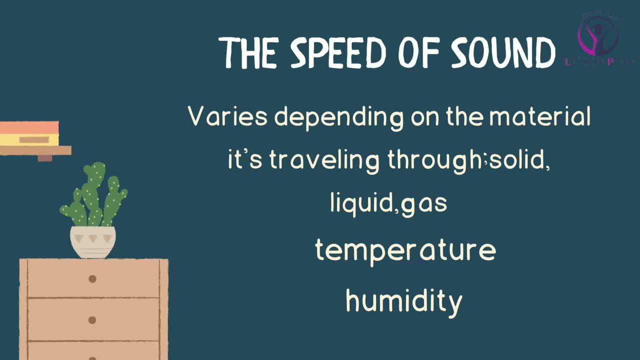 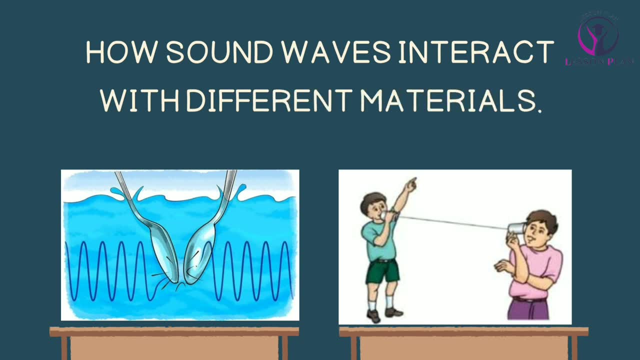 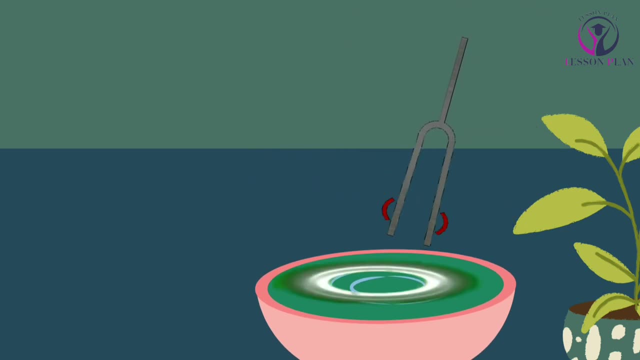 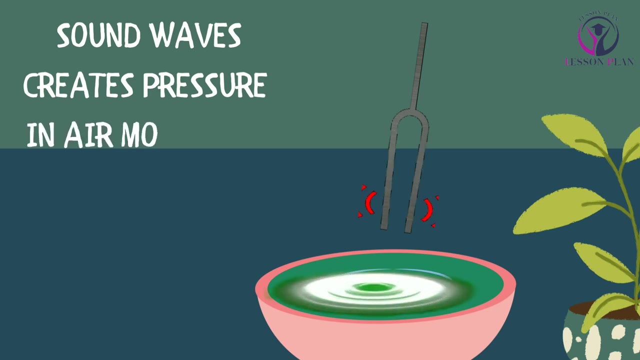 as other factors such as temperature and humidity. now let's explore how sound waves interact with different materials. sound waves can create vibrations in different materials and we can see this effect in action by using a tuning fork. a tuning fork is a small metal instrument that vibrates at a specific frequency when struck. if we 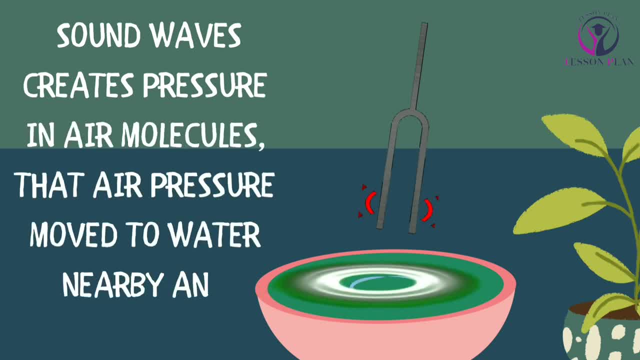 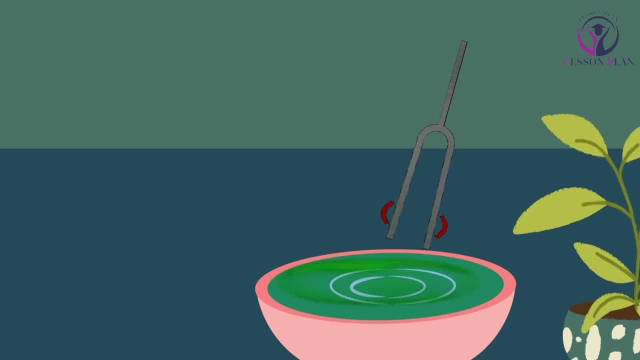 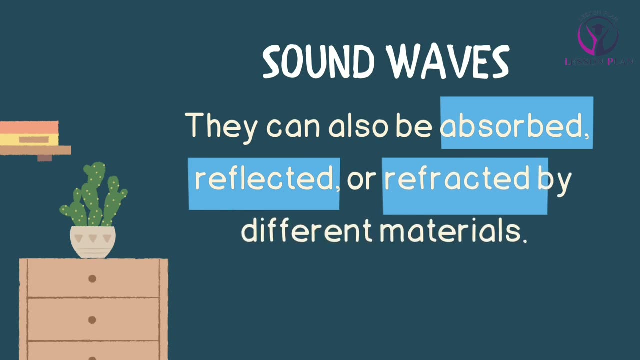 hold a tuning fork above a water surface, the sound waves from the fork will create ripples in the water, demonstrating how sound waves can create vibrations in different objects. but sound waves don't just create vibrations. they can also be absorbed, reflected or reflected by different materials when 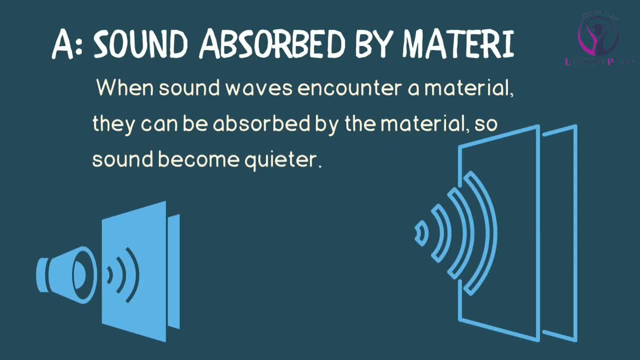 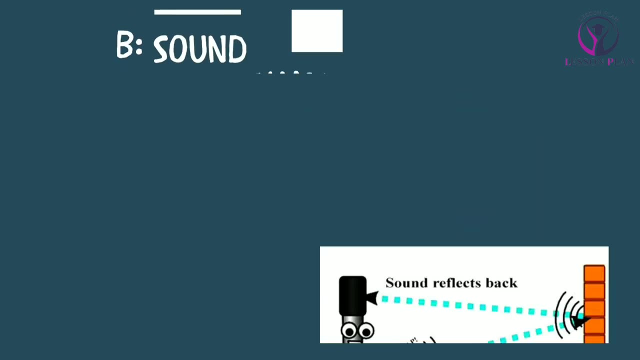 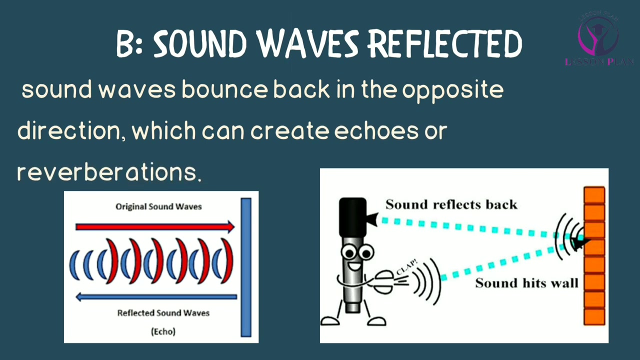 sound waves encounter a material, they can be absorbed by the material, which can cause the sound to become quieter. this is why sound is often muffled when we are in a room with soft absorbent materials like curtains or carpets. on the other hand, sound waves can also be reflected by certain materials such as hard surfaces like. 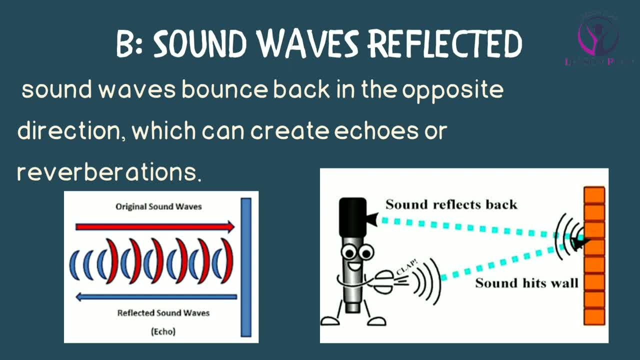 walls or floors. when sound waves are reflected, they bounce back in the opposite direction, which can create echoes or reverberations. this effect is often used in concert halls or music studios to create a more immersive sound experience. Sound waves can be refracted when they pass through different materials with different 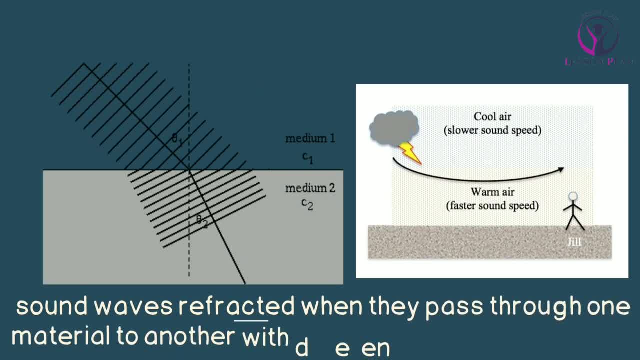 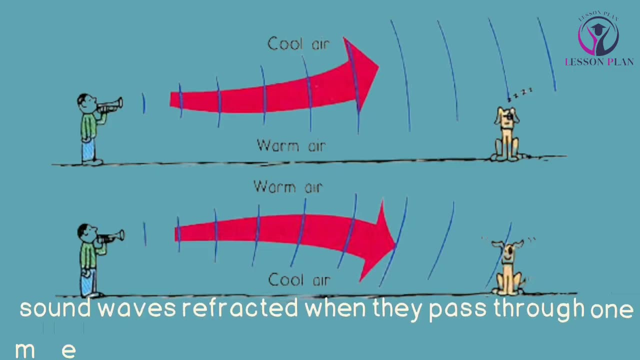 densities. Refraction occurs when the direction of a sound wave changes as it passes through a medium which can cause a sound to be distorted or muffled. This effect is often seen when sound travels through the atmosphere, where the temperature and humidity can cause sound waves to bend and refract. 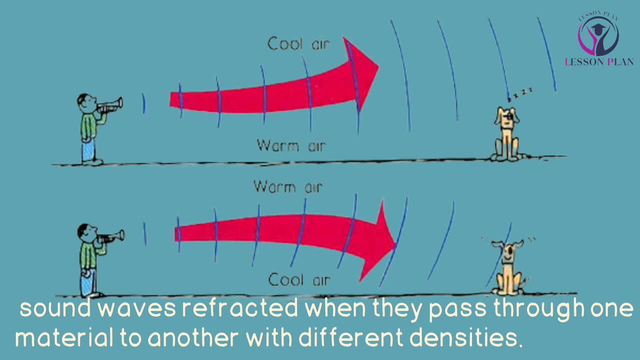 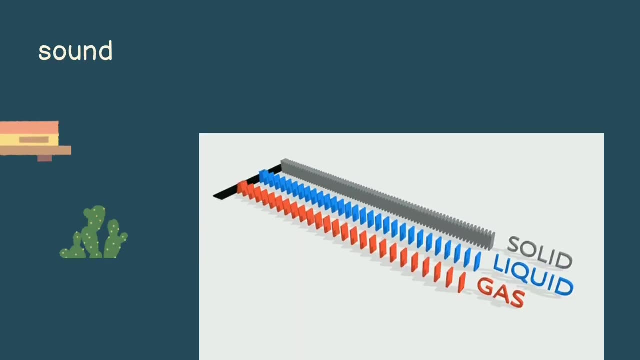 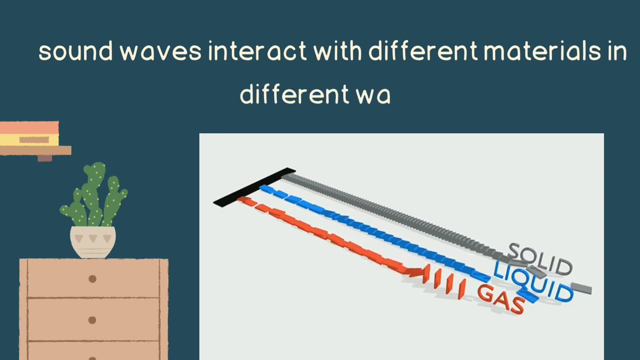 So, in summary, sound waves interact with different materials in different ways. they can create vibrations, be absorbed or reflected, and even be refracted as they travel through different mediums. Now we will conduct some fun experiments to help illustrate the concepts we have learned so far. 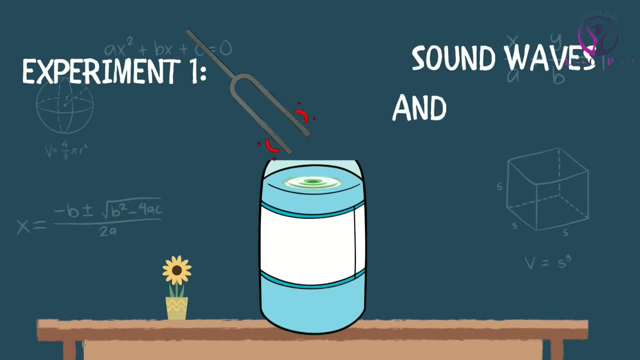 Experiment 1 is about sound waves and vibrations. For this experiment you will need a tuning fork and a plastic water bottle. First, fill the water bottle with enough water to cover the bottom, but not too much that it spills out when the bottle is tilted. 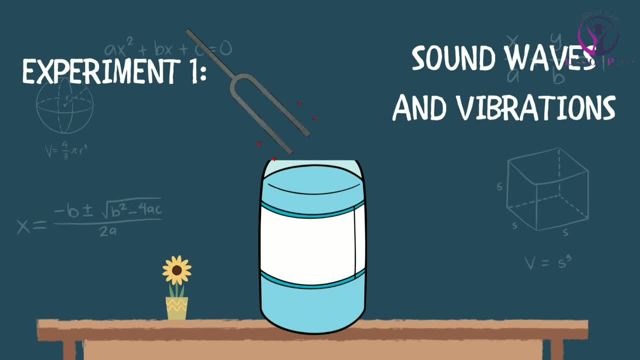 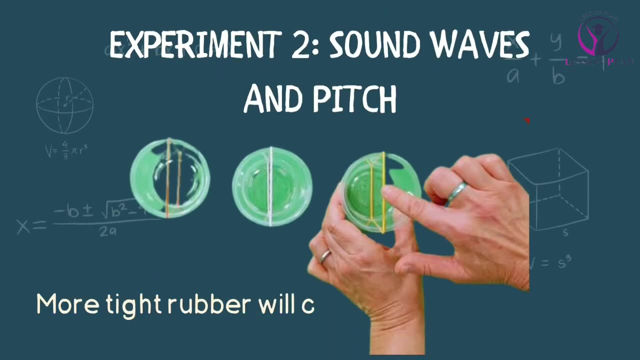 Then hold the tuning fork above the water and strike it against a hard surface. You should see ripples forming on the water's surface, showing how sound waves create vibrations in different materials. Experiment 2 is about sound waves and pitch. For this experiment you will need a rubber ball. 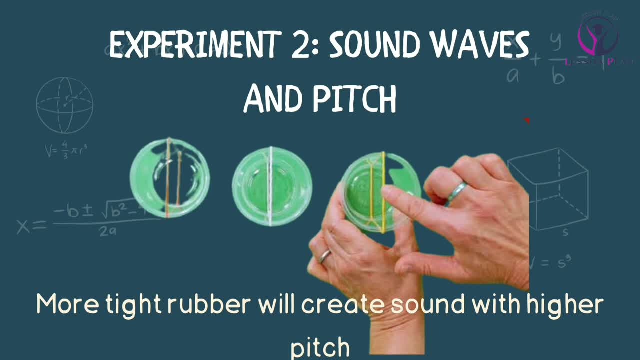